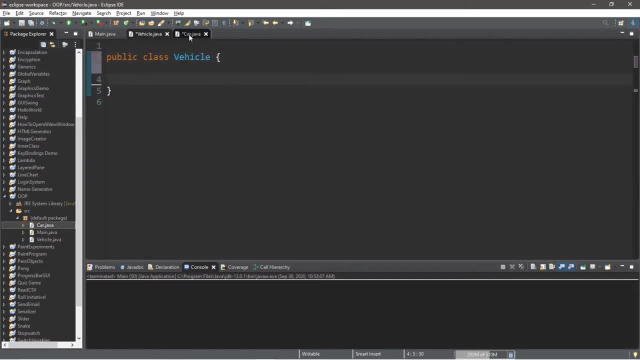 I have two additional classes, a class called vehicle and a class called car that extends vehicle. So car is the subclass, also known as the child class, of the vehicle class, and we can create objects from both of these classes, And let's try that. So first let's 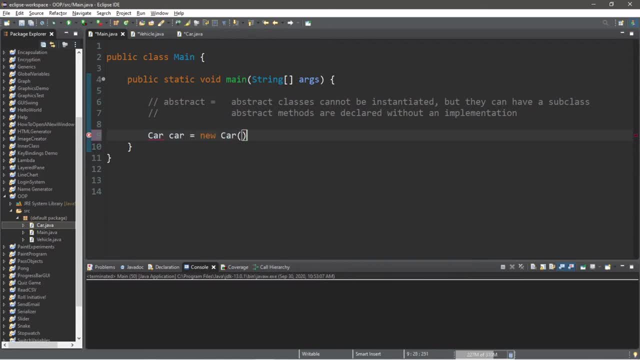 create a car, Car. car equals new car. And let's also create a vehicle object, because we can. So vehicle vehicle equals new vehicle. So we can create instances of both of these classes just fine, but we may not want to be able to do so. So, adding the abstract keyword to a class. 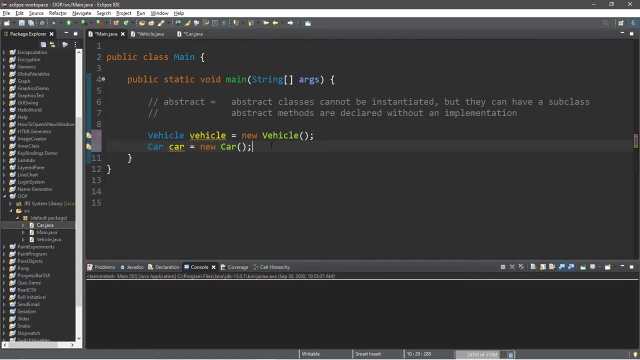 adds a layer of security. So here's an example. Let's pretend that we walk into a car dealership and we ask a salesperson for a vehicle and they might reply with: well, what kind of vehicle are you looking for? Are you looking for a car? 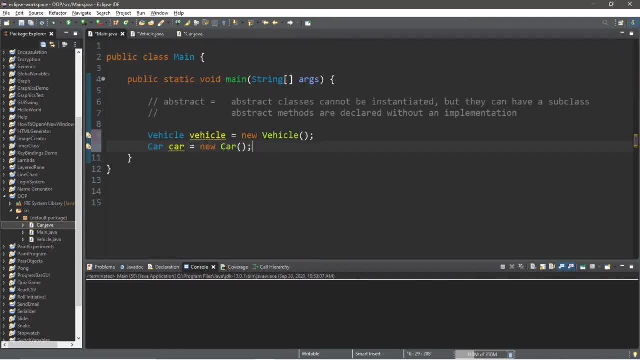 a motorcycle, A truck, And we just say, no, we want a plane, generic vehicle. and they might think you're crazy, because a vehicle is too generic. Then it might say it's abstract. well, at least it should be abstract. We need a certain type of vehicle. So what? 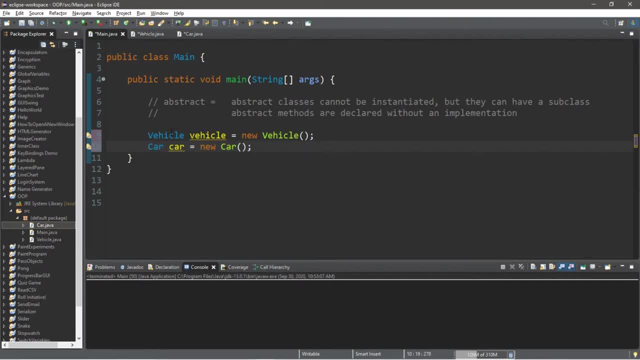 we could do to prevent somebody from creating an instance of a class that is too vague or abstract. we can use the abstract modifier when we declare this class. So with vehicles, let's add the abstract modifier So I can use vehicle to call an example of this type of vehicle. When they determine if 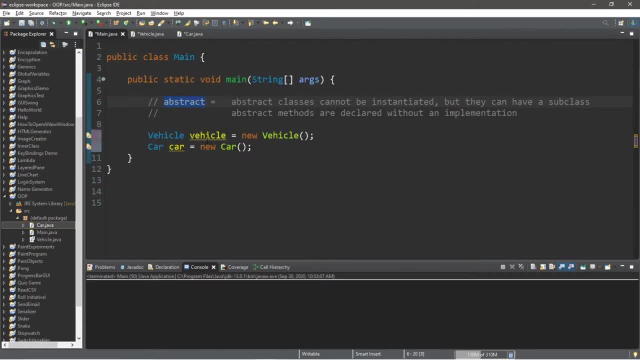 it is abstract modified or abstract modified by party. I can put them on my any type of vehicle. I can start creating an instance and label they that are too vague or abstract, I can use the abstract modifier- So what modifier? and we can no longer create an instance of this class and it says: cannot instantiate the 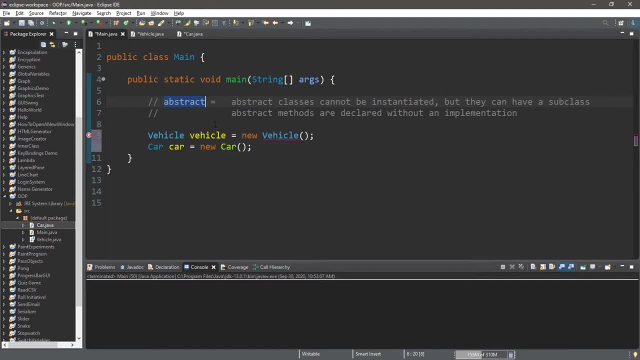 type: vehicle. so this adds a layer of security to this program. so in order to get this to run, we cannot declare a vehicle object. we have to pick a certain type of vehicle, a child class of the vehicle class, whether it's a car, a bike, a truck, whatever. now we can also create an abstract. 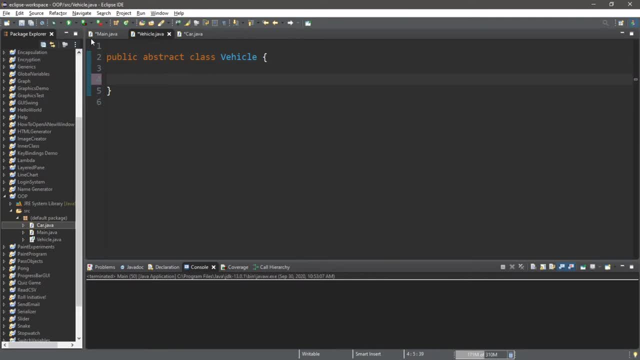 method too. so let's declare this within the vehicle class, and an abstract method is declared without an implementation, so that means without a body. so let's say that all vehicles should have a method to go, because that's the point of a vehicle. so all vehicles should go. this is going. 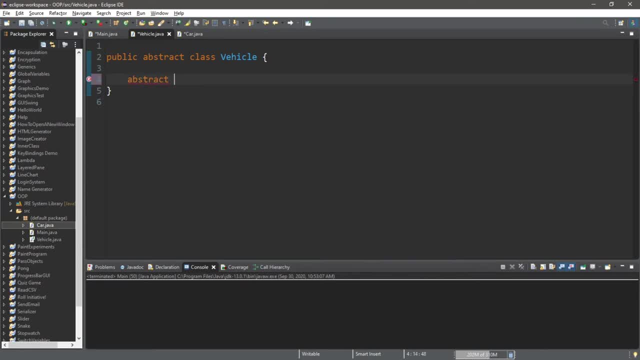 to be an abstract method. we're going to use the abstract keyword. we need a return type. we'll just make this void and this will be go, and we do not need a body for this method. and if we attempt it, we're going to get a body for this method. and if we attempt it, we're going to get a body for. 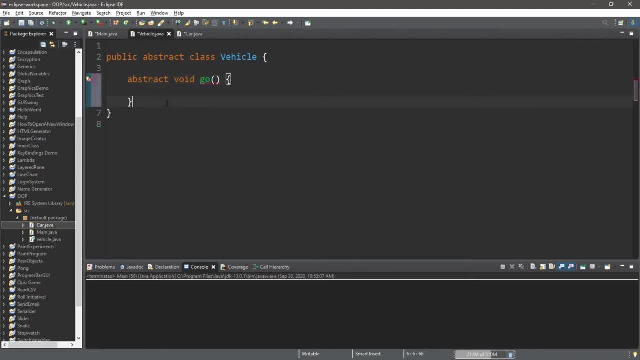 this method and if we attempt it, we're going to get a body for this method. and if we attempt, add a body, a set of curly braces, well, we're going to have a problem. and this says abstract methods do not specify a body. so what this does is that it forces us to implement this method in one of 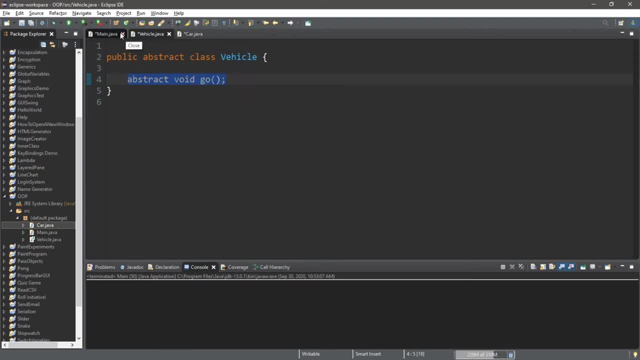 the child classes that our vehicle class has. so if we attempt to run this actually you can see that it's popping up already. the type car must implement the inherited abstract method vehiclego. so what we could do is add unimplemented methods, and what we're doing is actually method overriding. 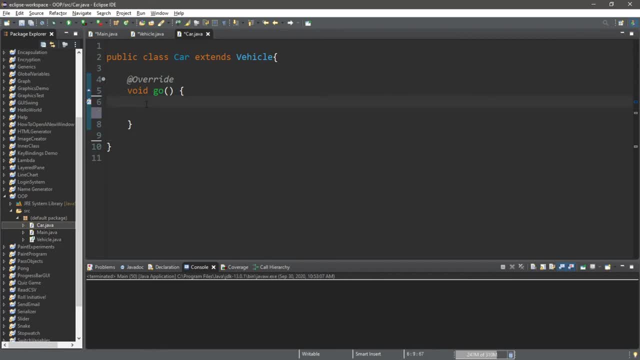 so we can add our own implementation of this go method more specifically for cars. so let's say, maybe the driver is driving the car and that should be fine. so we can no longer create an instance of the vehicle class because it's abstract and a vehicle object is too vague. so we would like 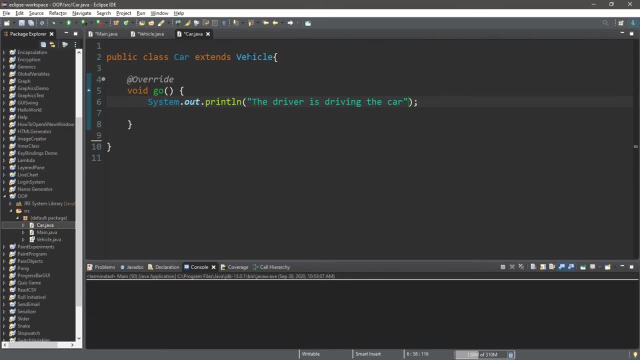 to force a user to run this method in one of the child classes that our vehicle class has. so we can also use the go method that is found within the vehicle class too, but we are forced to override it or implement it in each of the child classes that our vehicle might have, and it's just the same. 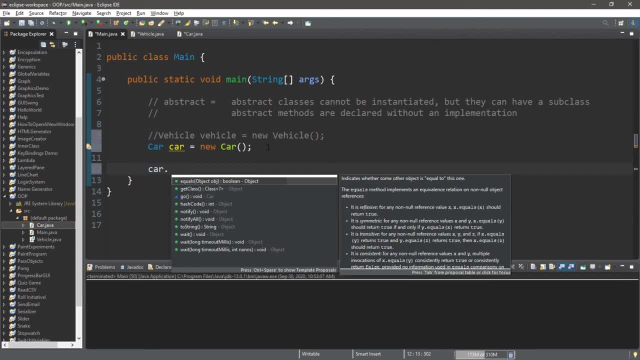 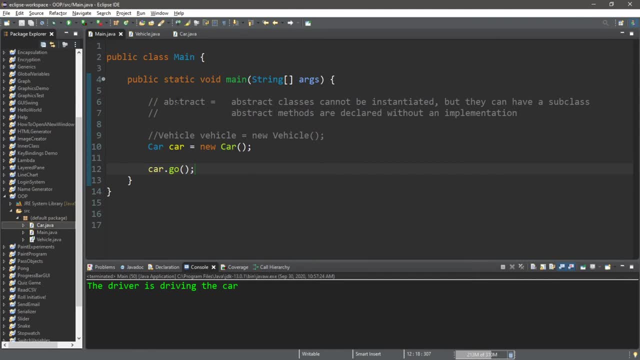 as what we would normally do with calling a method, so cargo, and this will print: the driver is driving the car. so that's the whole point of the abstract keyword. it adds a layer of security to your program and this will print: the driver is driving the car. so that's the whole point of the abstract. 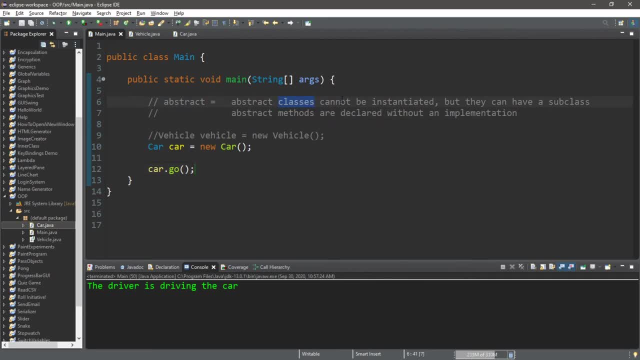 this can be applied to both classes and methods. if it's applied to a class, a user cannot instantiate an instance of an abstract class, and with abstract methods they are declared without an implementation. but a subclass or child class has to implement that somewhere. well, that's the.